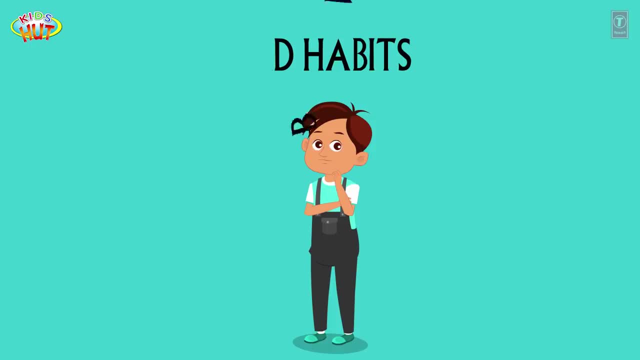 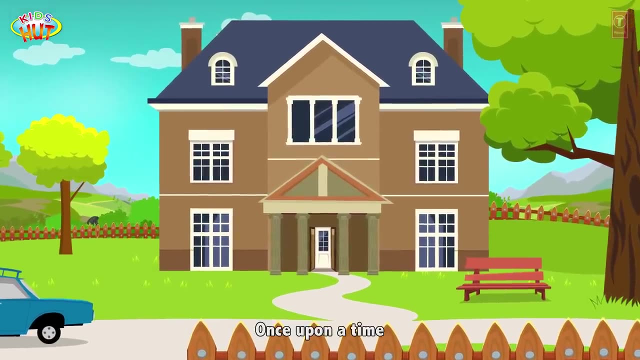 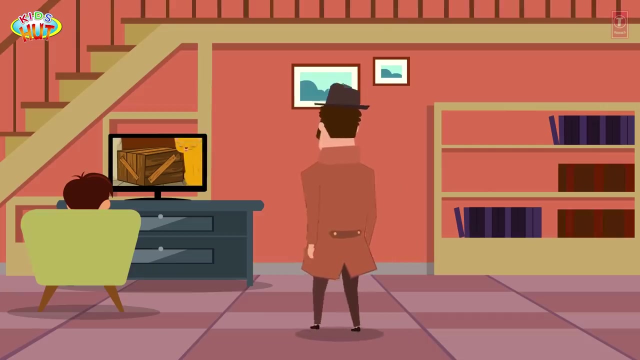 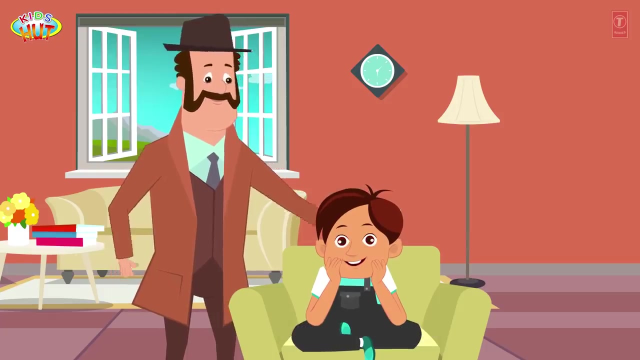 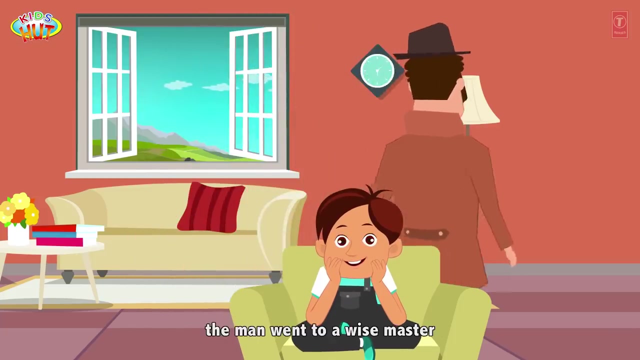 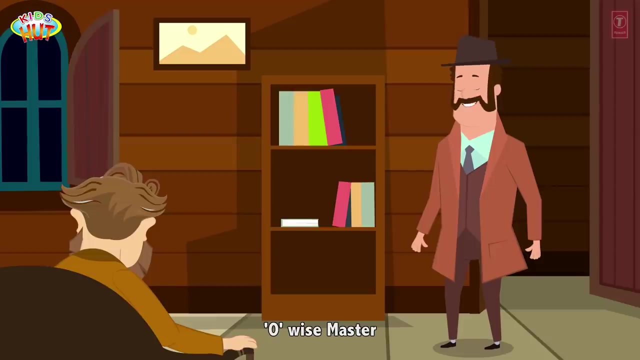 Bad Habits. Once upon a time a rich businessman lived with his eight-year-old boy. The businessman loved his son but hated that he had some bad habits. Worried about his son's behaviour, the man went to a wise master. Oh, wise master. 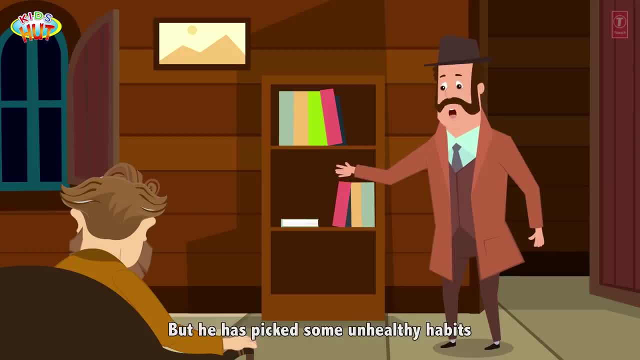 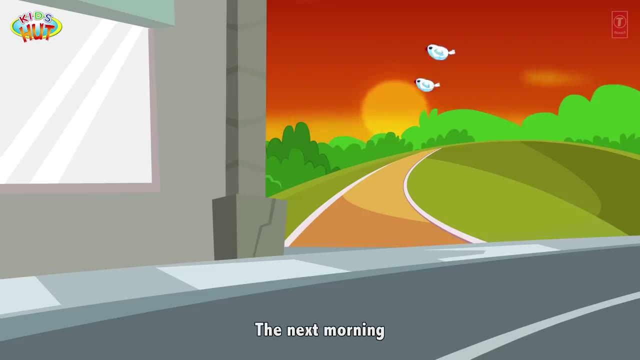 My son is a very good boy, but he has picked some unhealthy habits which I cannot get him. I don't want him to let go. I worry about him all the time. Please help me, Bring him to me tomorrow morning. The next morning the man did as the master had said. 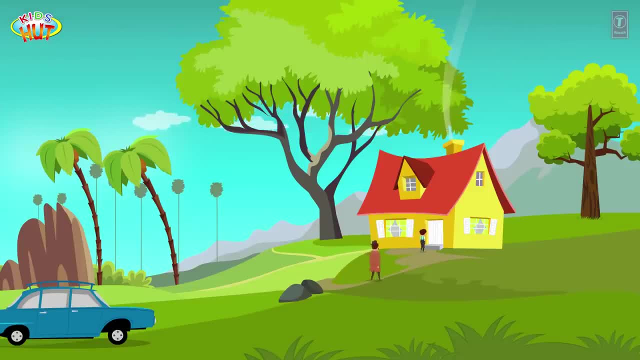 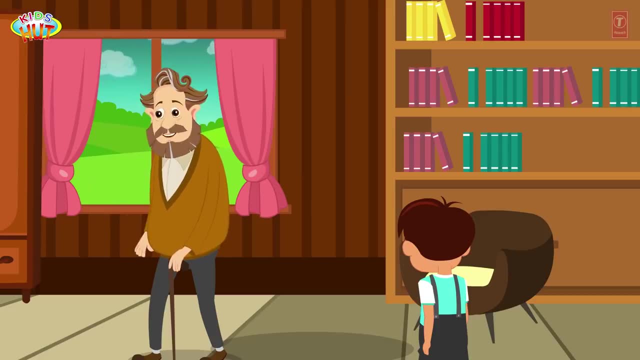 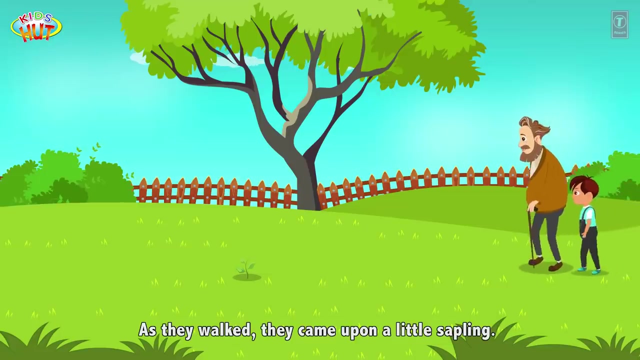 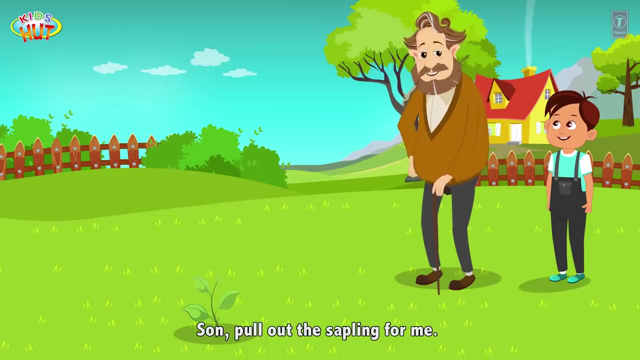 He brought his boy to him. Come, son, Let's go for a walk. The boy obeyed. He went for a walk in the garden. As they walked they came upon a little sapling. Son, pull out the sapling for me. 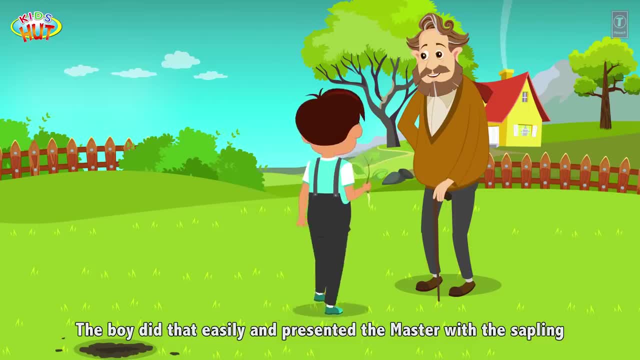 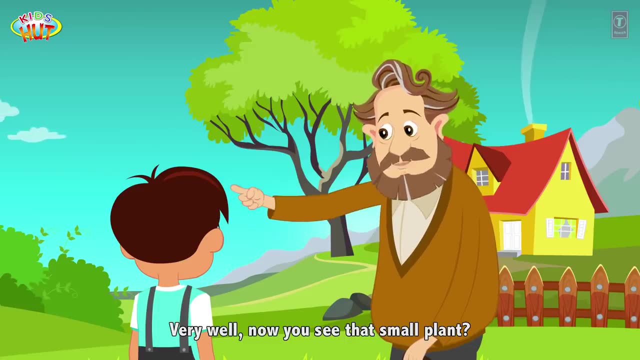 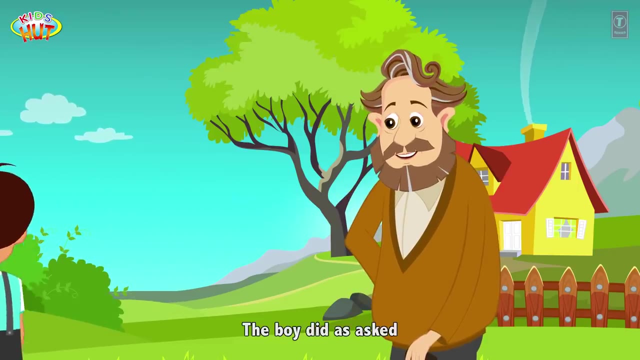 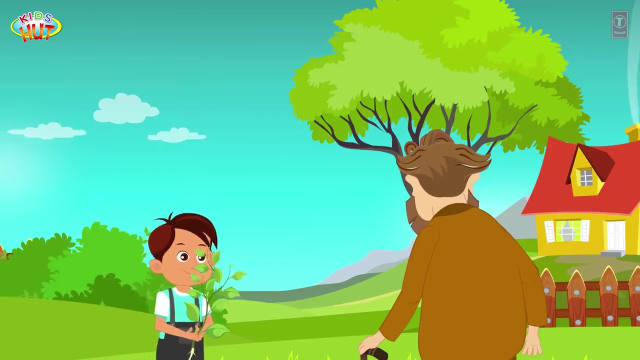 The boy did that easily and presented the master with the sapling. Very well, Now you see that small plant, Pull that out for me. The boy did as asked and easily pulled the plant out. Next, the master asked him to pull out a bush. 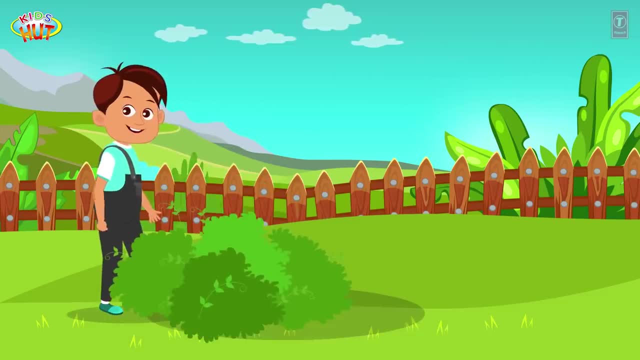 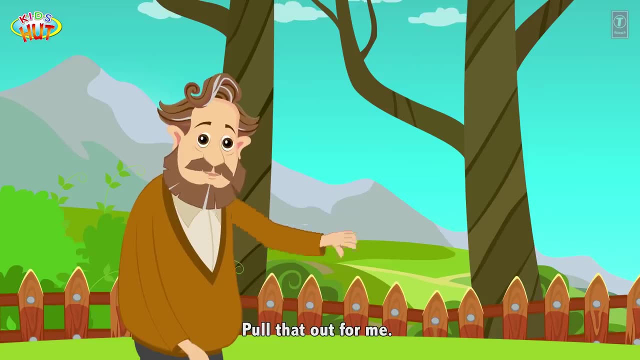 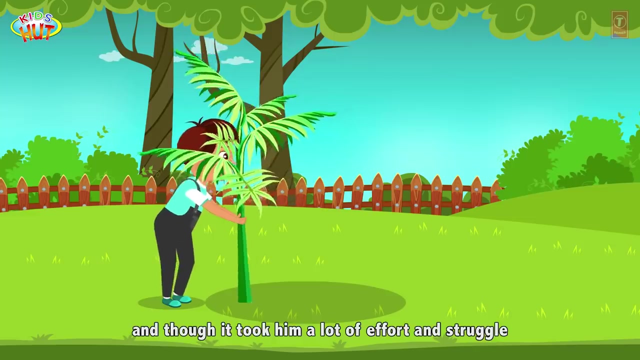 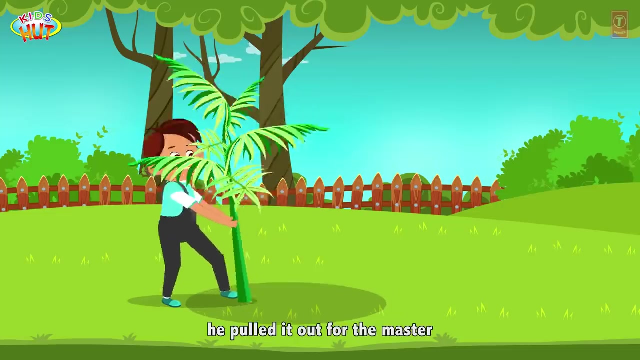 It took some effort, but the boy did that too. Now see that small tree, son, Pull that out for me. The boy went to the small tree And though it took him a lot of effort and struggle, he pulled it out for the master.